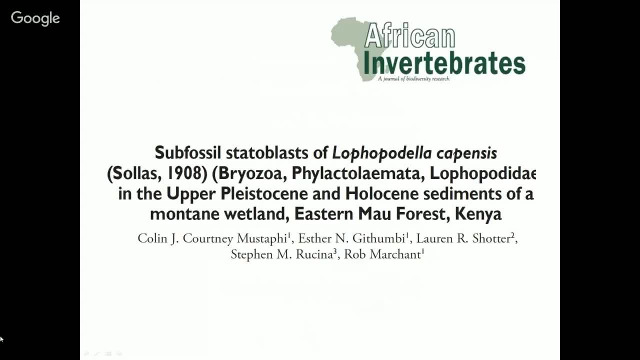 It's sort of an opportunistic. It's a paper where we're doing some work on a sediment core collected in eastern Mao and we came across something quite interesting in the sediment, which was the Stadoblast, which is a reproductive part of a freshwater bryozoa. 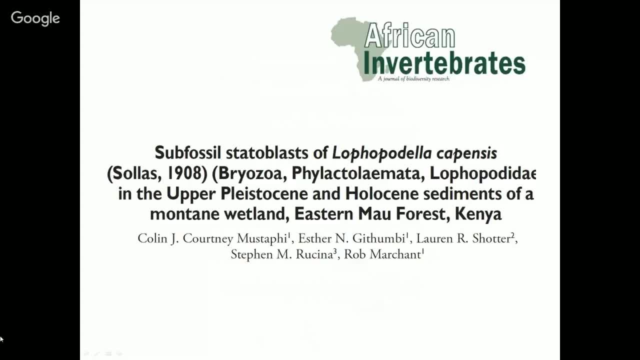 And what we found curious is that a few years ago, or a decade or so ago, there was a WWF biodiversity survey and they did not find any bryozoa at the site. So looking at it through the historical perspective, we found that there was no bryozoa at the site. 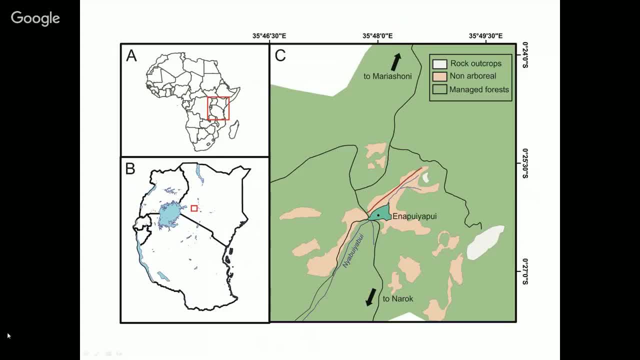 So, looking at it through the historical perspective, we found that there was no bryozoa at the site, And the personal perspective was quite curious. So the site is in western Kenya, in the Eastern Mao Forest, and it's just a small wetland in a industrial forest. 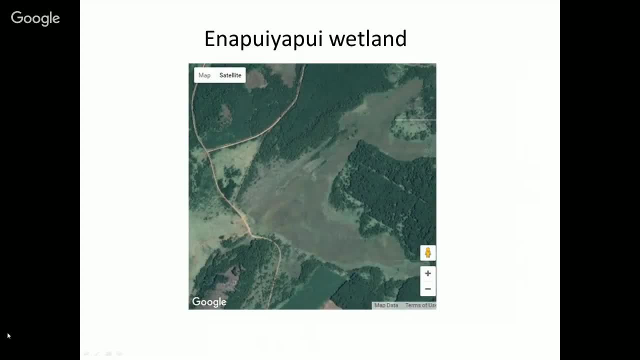 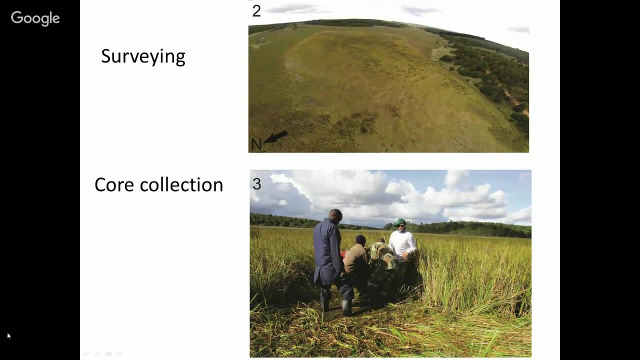 So this is just the Google Earth view of it, and this is the swamp area in here, and then just a small drainage this way, And so it's surrounded by planted tree stands that are managed by a Kenya Forest Service. So in 2014,, Esther and I led a crew up there to core the swamp. 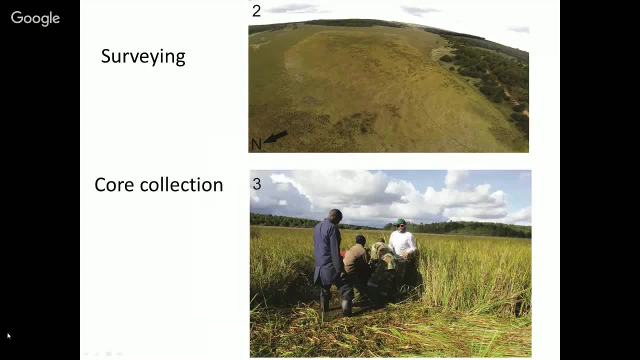 So it's full of grass and cypressia. The water level is quite low. at the time we were there, I think it's around 30 centimeters worth of water. There wasn't very much open water at all. It was very overgrown. 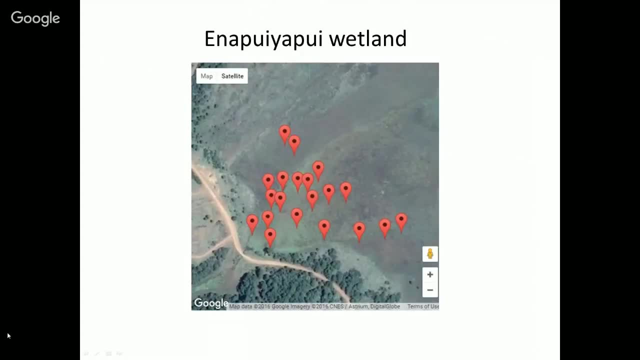 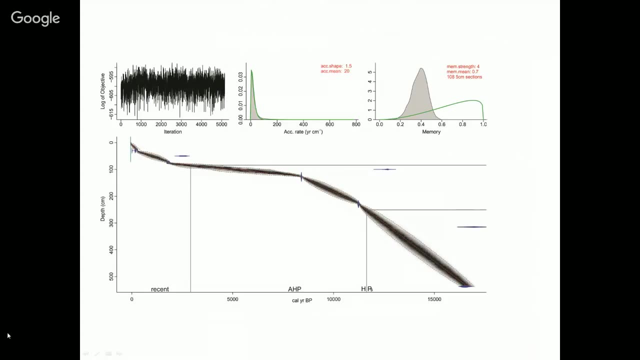 Then we surveyed surface samples of sediment all across the swamp and we also took a core from the center of the swamp and we've had some radiocarbon dates collected on that. It built a preliminary age model and so the core actually goes down about five and a half. 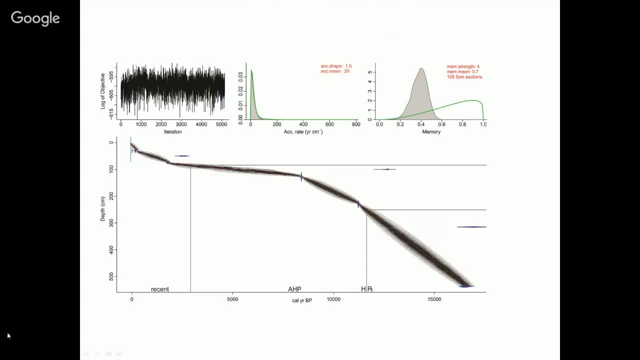 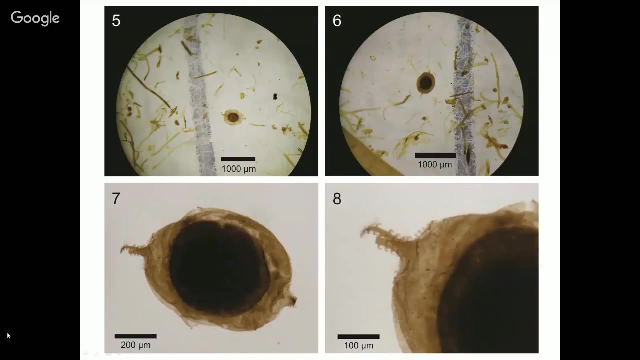 meters and it dates to about 16,000 years ago. so it captures that transition from the Pleistocene to the Holocene and throughout the African humid period, as well as some into the recent past. Okay, And so during investigation of this core, I was counting some charcoal and we came across. 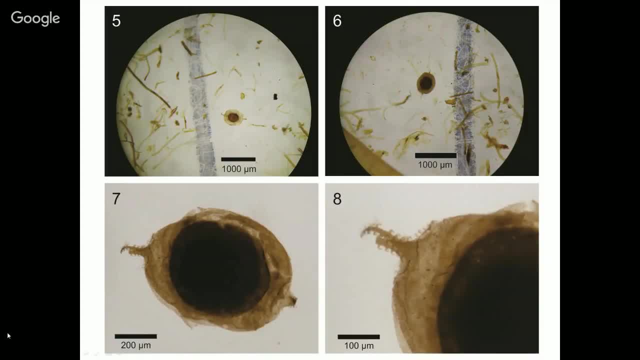 this thing. So at first I didn't know what it was. It's a chitinous, very small, 300 microns size romaine, but it was readily identifiable to a single species, Lophopadela capensis. and what's really interesting about this? 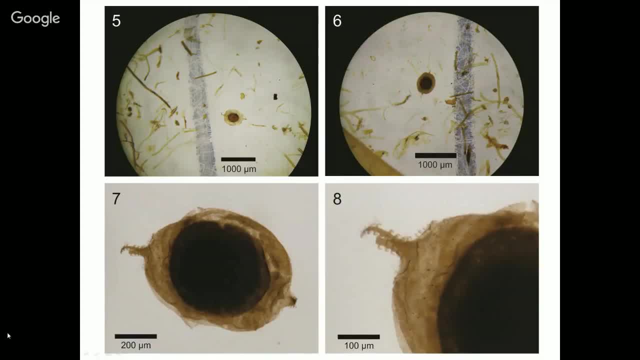 species is that it's only found in about six locations currently- Okay, So primarily in South Africa, another site in Kenya and recently in Israel, which is a curious pattern. So that's what it looks like, And so it was found in a few locations down the core. 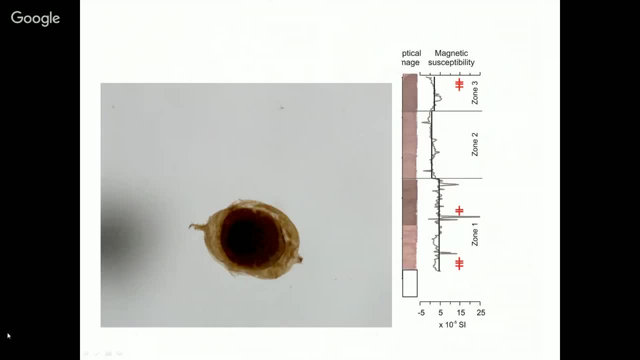 So that's the top of the core and this is an image that Esther collected at the University of the Core phase and magnetic susceptibility values. But primarily this is the rest of the core. Okay, So this is. the red pluses are the locations of where the fossil was found. 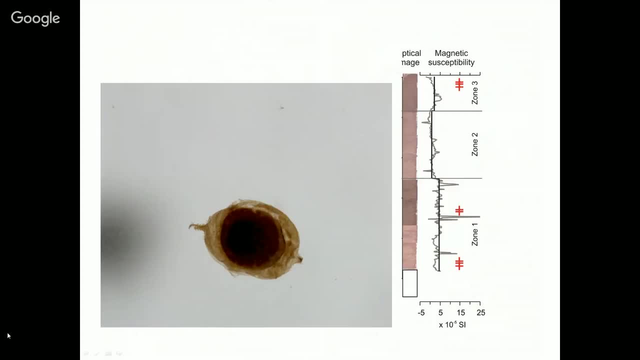 And so it was found throughout the record intermittently It's just presence data for the taxa, but curiously it was in the very recent past, in the past few hundred years, but not observed today, And so I think that sort of drove the impetus for just writing a quick note on this occurrence. 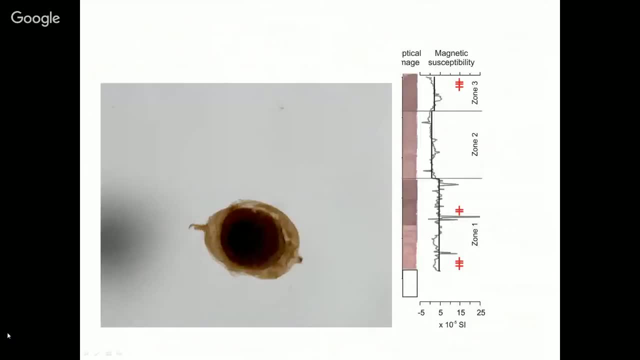 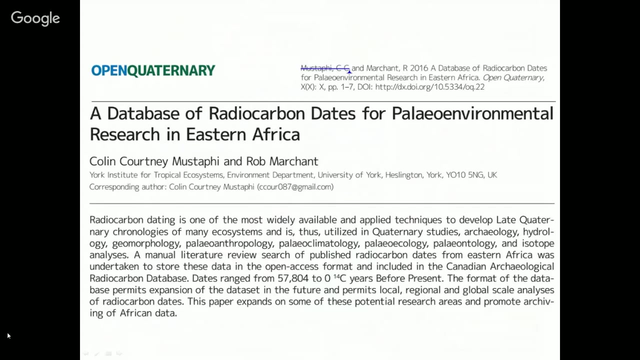 And I guess it fits into the sort of biodiversity Aspect of what this type of data can provide insight for. So this is just another note that we recently published. also, I guess throughout the time of surveying the literature in East Africa, we collected all the radiocarbon dates that 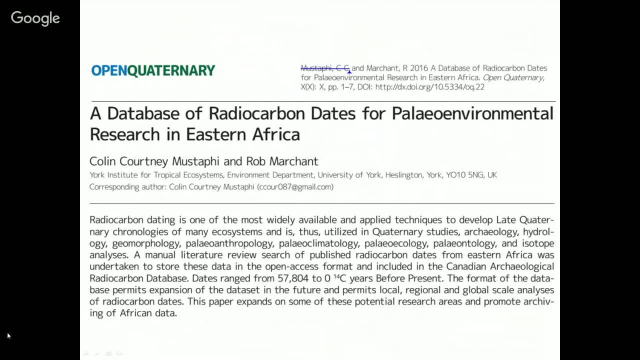 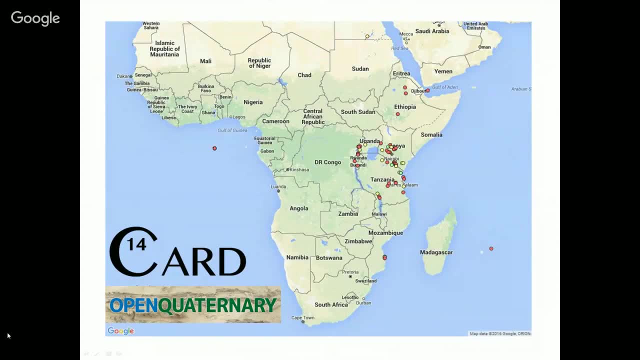 were published and we've been putting them into a database that's freely available. So it's the Canadian Archaeological Radiocarbon Database. It's a global database, Although the name doesn't sound like that, And all radiocarbon databases that are available currently have a lack of data in Africa wide. 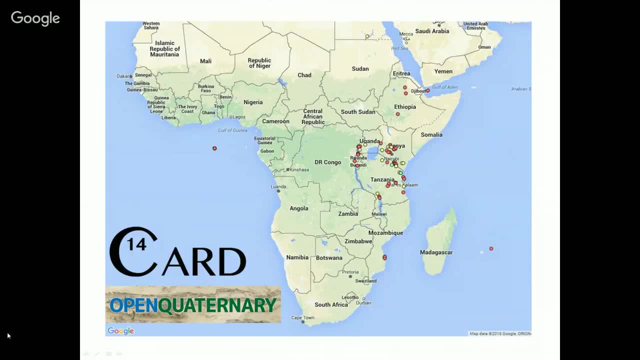 So these are the first actual African dates to be submitted to an open access database for people to use, And it's a live database that can be updated continuously and added to, And so, if you're interested in these types of tools, it collects radiocarbon data dates. 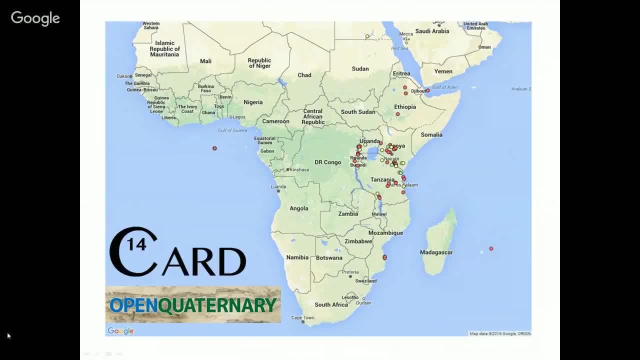 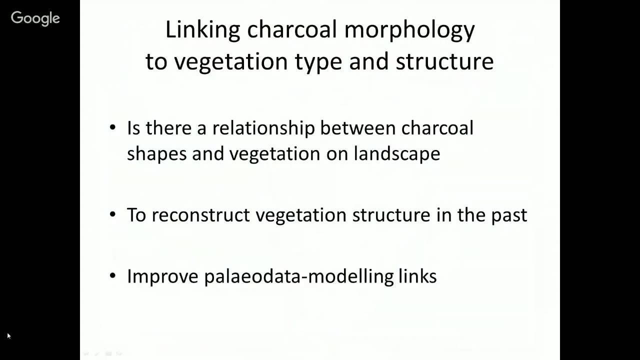 from archaeological sites, geologic sites like we have been working in, and also from paleontological remains as well, So that's another tool that's available if you're interested. Primarily, a lot of the ongoing work that I'm active in is looking at charcoal in these. 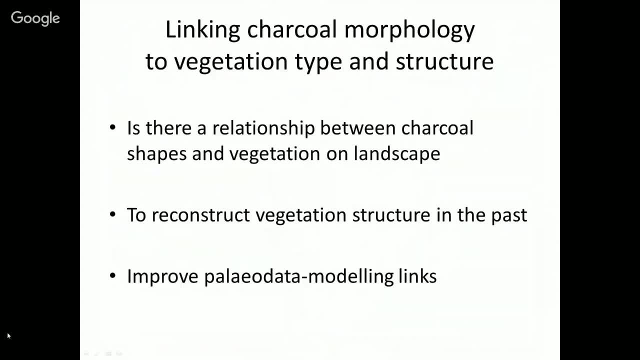 sediment records, to think about fire activity in the past and start to think about how to use different metrics Or maybe in new approaches to link the data that we can collect to relevant ecological and conservation questions, And also thinking about human and environment interactions throughout the past. 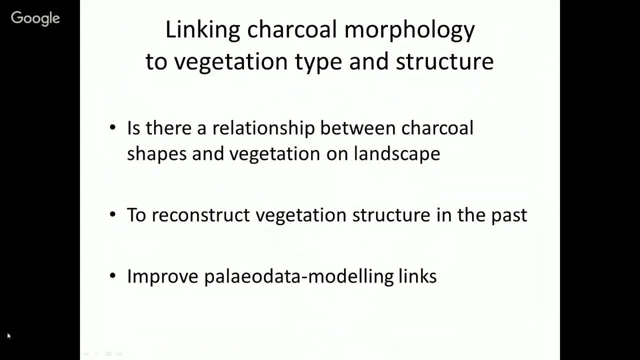 So one research question that I'd like to pursue is looking at the relationship between the morphologies of the charcoal, the different shapes that are present in the sediments, and trying to link that to the composition of the vegetation. Okay, So the morphologies of the vegetation as well as the structure of it. 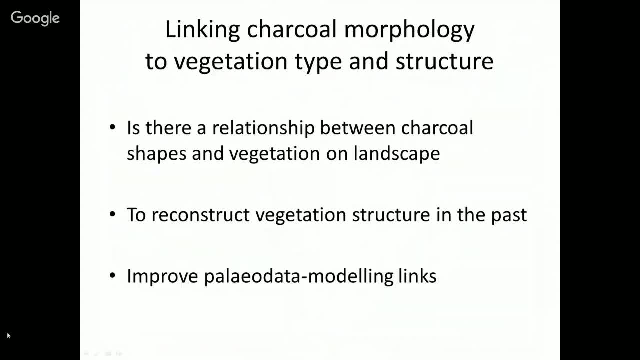 So the arrangement is it just grasses, grasses and trees or trees And the distribution of those around a site And if that's possible to do that quantitatively, it might be possible to reconstruct the structure of the vegetation at the site through time. 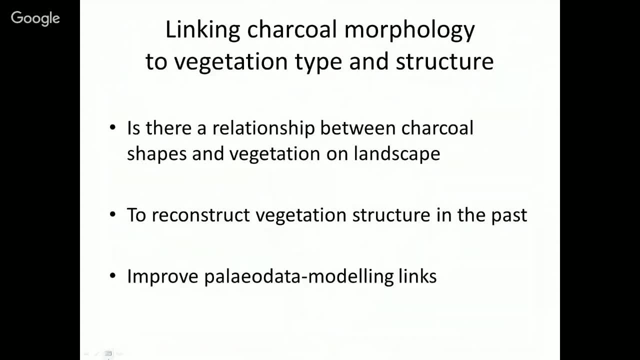 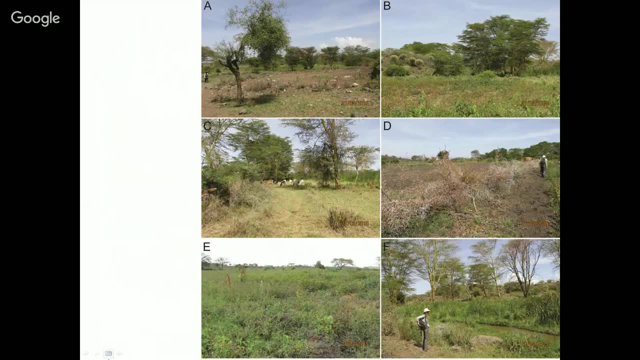 And that should be able to improve linkages between the type of paleo data we're able to collect and land coverage. So there's a quite diverse range of land cover types and structures that are seen, and these are actually just snapshots from the Amboseli area only. 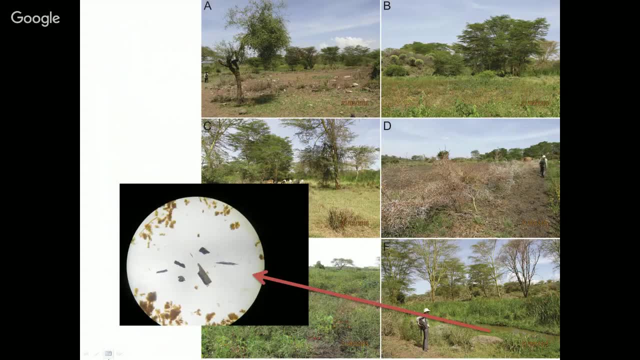 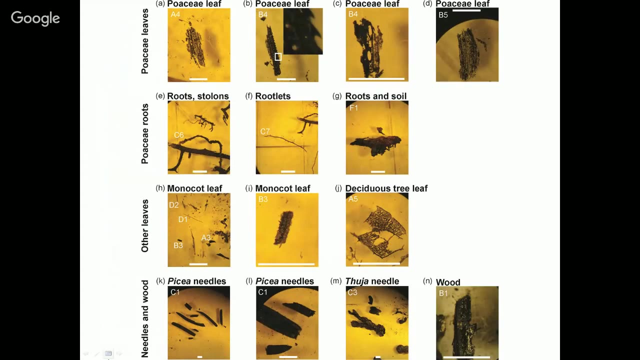 And you can see there's quite a diversity, And so when we collect sediment from these different locations, there's an assemblage of charcoal morphologies that are present, And so there's quite a range of different types of sediments. So we're able to experimentally link those to different plant parts and different plant. 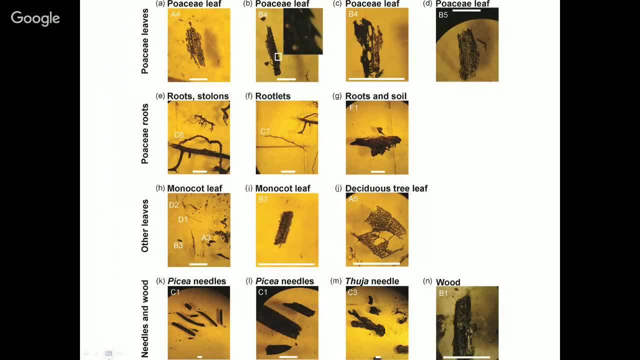 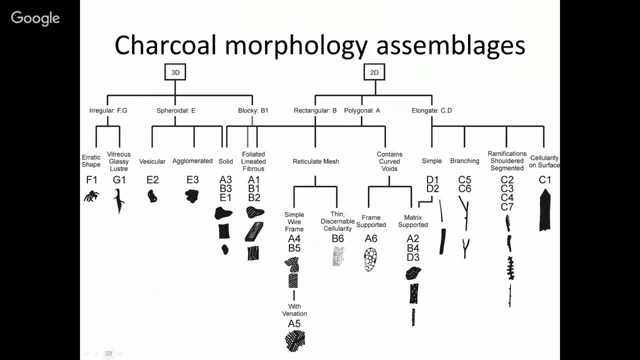 types that are present on the landscape, And if we classify those, then as we count the charcoal in a sediment core, then we're able to build those assemblages through time, just like we would do for any other microfossil, And then we get lots of squiggly lines. 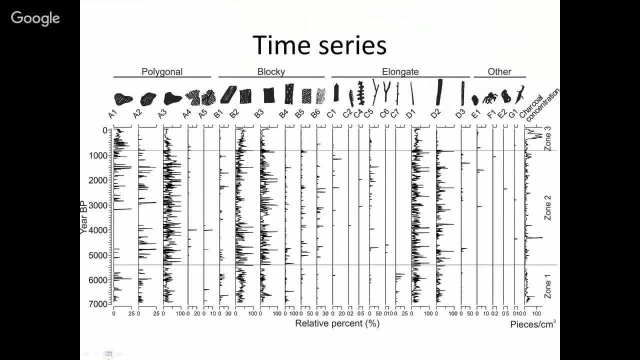 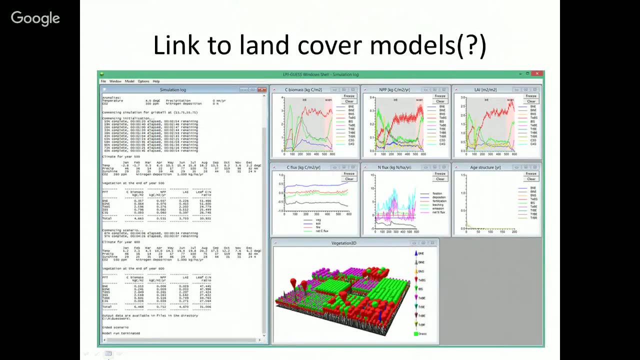 So this would be a sediment core with the recent at the top and the past at the bottom and the very variation in the charcoal assemblage or morphology assemblage through time, And then the ultimate goal would be to link that with land cover models, if that's possible. 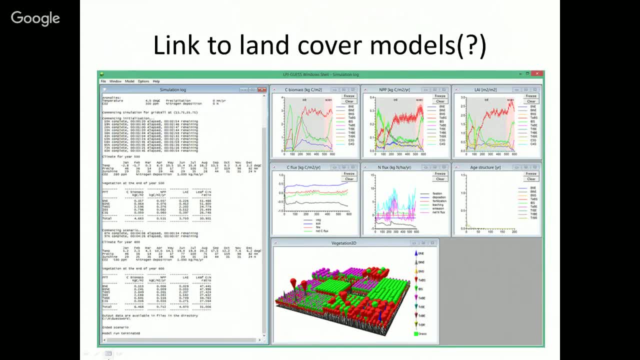 and so how to pursue that, And so some of the ongoing work is just collecting surface. So sediment samples from depositional sites across the world and a little bit I've been looking at also soil samples from East Africa to also look at how the charcoal is preserved. 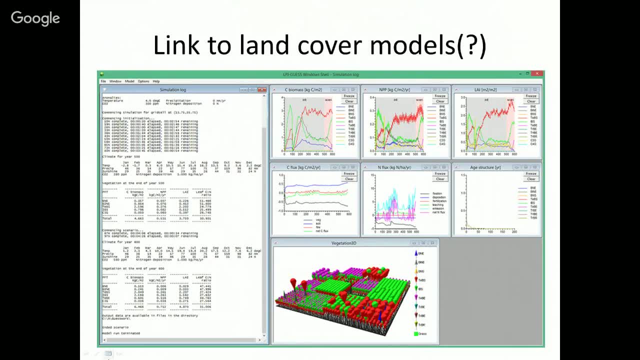 in there and if it does relate to the structure of the vegetation that's currently there. So once we have enough of this type of data and it's all will be freely available through the modern global charcoal database. Okay, Thank you, Thank you. 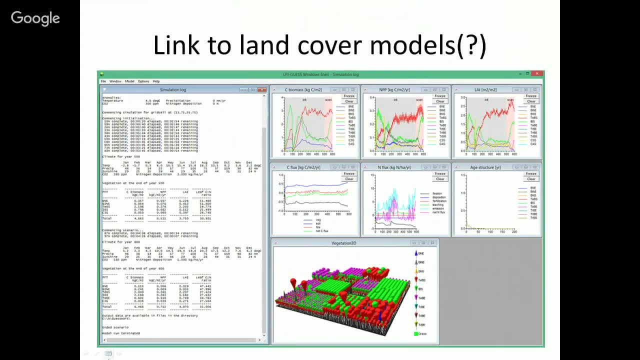 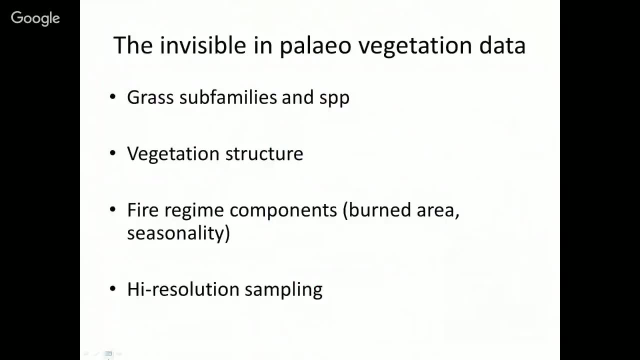 We hope to be able to build some quantitative links between those morphology assemblages and the structure and to see if this is actually possible. And something that comes up in a lot of the discussions that we have, I guess, is thinking about what is still invisible with the paleoenvironmental data that we're able to collect and trying. 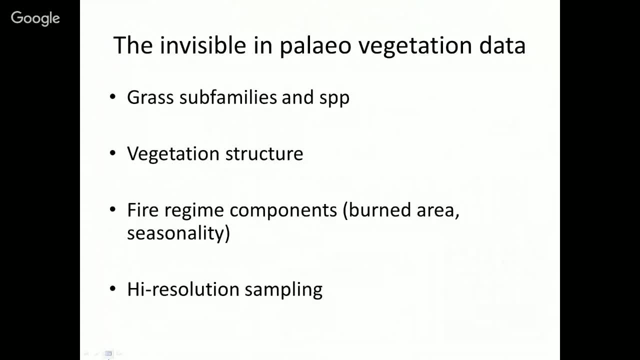 to think of ways of pursuing measurement of these in some capacity to sort of strengthen the links, And in the meantime we're trying to make sure that we're still able to get some of the data that we need in the space that we have. 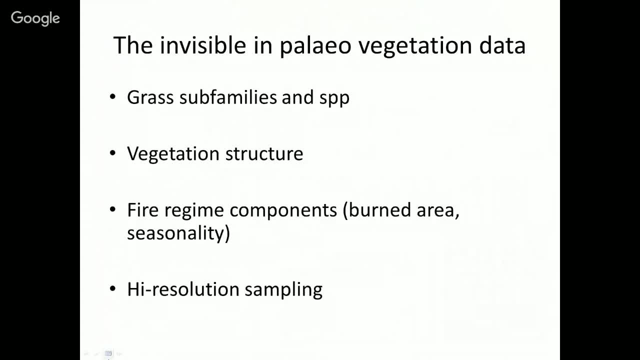 So I think this is a really interesting question that's been asked a lot lately in our research that we're trying to do in the context of this, because it's a very complex problem And so if we can sort of look at that and do some research in the context of this, 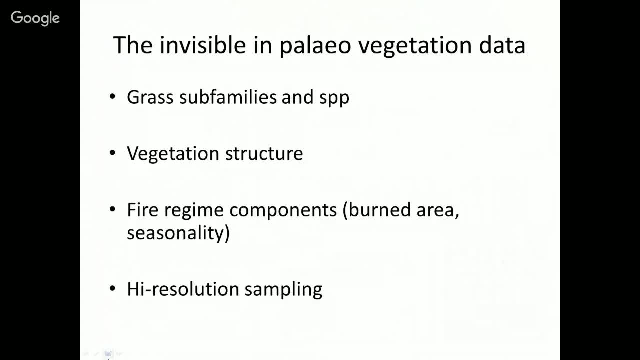 that's probably something that we can do. So I think that we're doing a lot of research on the question of how the environment can be used to measure the environmental impact of these models. And just quickly, this is a few that would be quite relevant and interesting in the